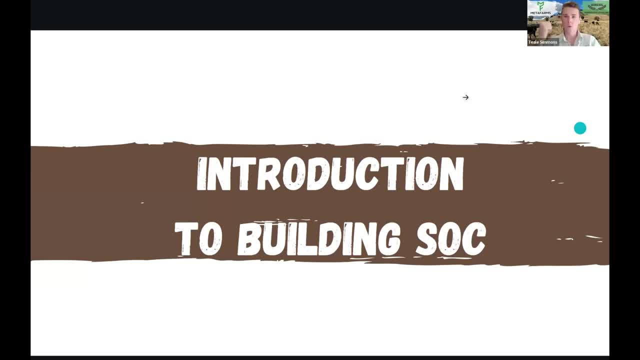 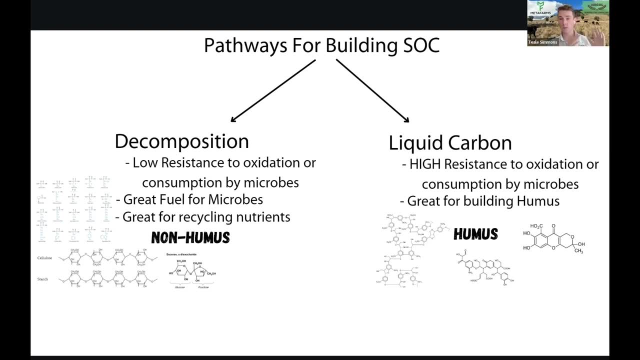 The two pathways for building soil: organic carbon. The first one is the decomposition pathway, which there's low resistance to oxidation or consumption by microbes, So this pathway is really good for creating fuel for microbes and it's great for cycling nutrients. Now, typically, this is a non-humus pathway, and so we're taking the building blocks of plants, which are all our non-humans, and we're converting them into the simple compounds. 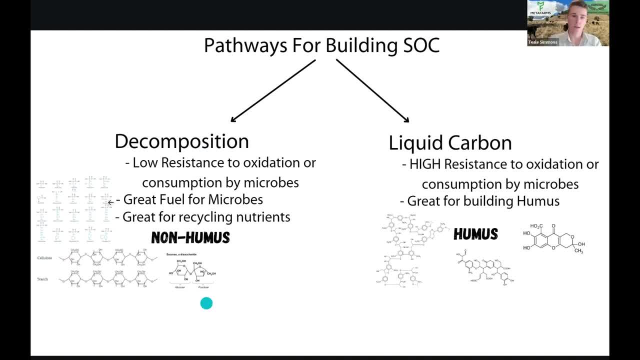 And so here we've got our carbohydrates, we've got our sugars, we've got our amino acids, all of those things. On the other side, we have our liquid carbon pathway. Now this is high resistance to oxidation or consumption by microbes, and it's great for building humus. 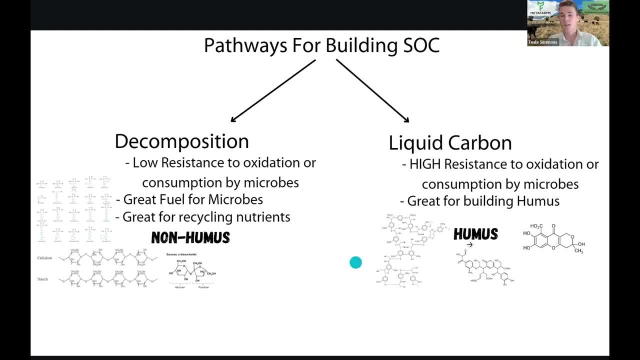 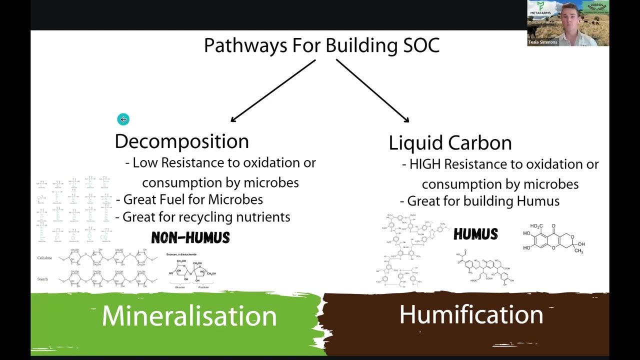 And so we're going to get these structures. It's very important that we look at liquid carbon pathway closely so that we can really understand how we can build soil, organic carbon, effectively, Effectively. So another I guess terminology for the decomposition pathway is mineralization and for the liquid carbon pathway that's called humification. 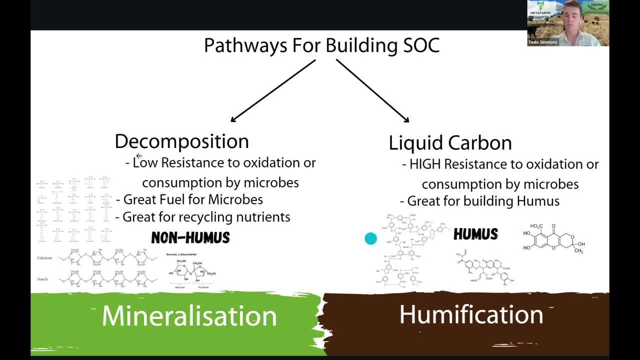 So decomposition and carbon produced from that typically lasts from months to years And that's why scientists have historically said it's really hard to build soil organic carbon and it takes thousands of years to build because they've been looking at it for years. 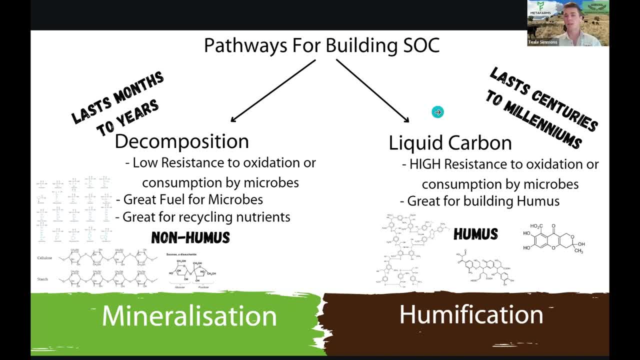 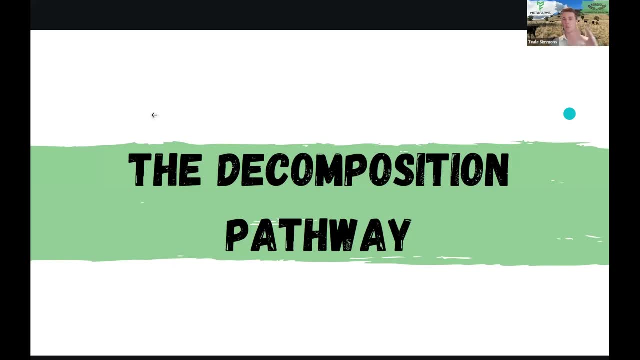 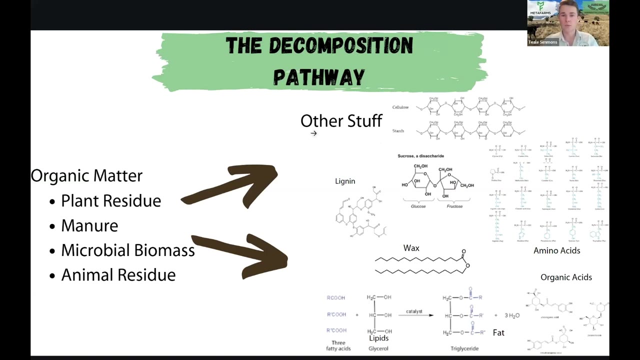 So this decomposition pathway, whereas in our liquid carbon pathway, the humus lasts for centuries to even potentially millenniums, so a long, long time. it's very resistant to breaking down. So let's have a look at decomposition pathway. This is effectively having organic matter, so our plant residues, the manures, microbial biomass, as well as animal residue. 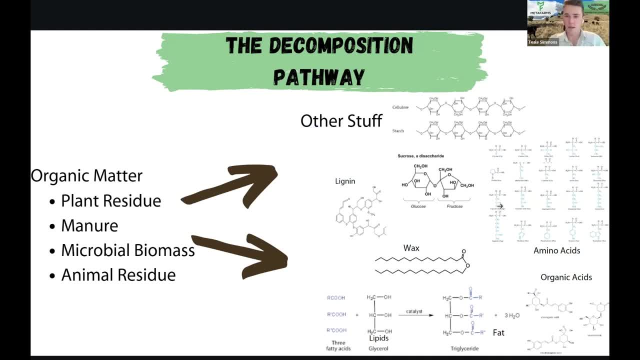 That's going to break down to produce all this other stuff That's going to break down to produce all this other stuff. So we're going to have our amino acids, organic acids, our fats, waxes, carbohydrates, simple sugars. you know, all of that stuff is going to really break down. 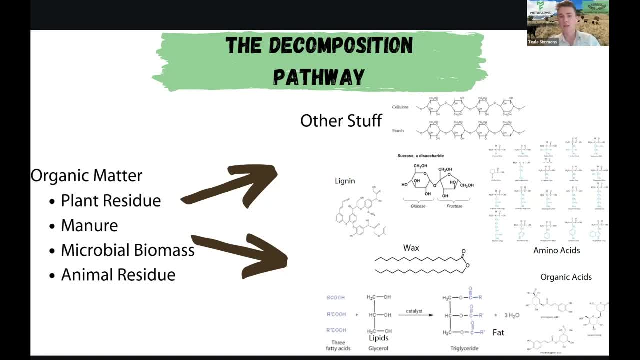 So we're going to have our amino acids, organic acids, our fats, waxes, carbohydrates, simple sugars. you know all of that stuff is going to really break down. So we're going to have our amino acids, organic acids, our fats, waxes, carbohydrates, simple sugars. you know all of that stuff is going to really break down. 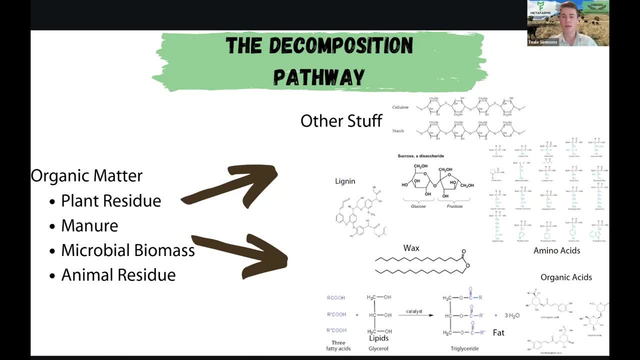 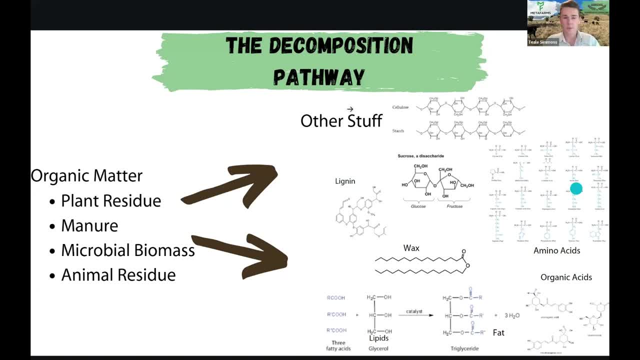 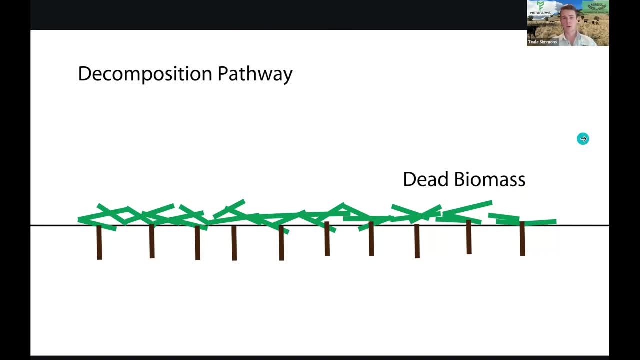